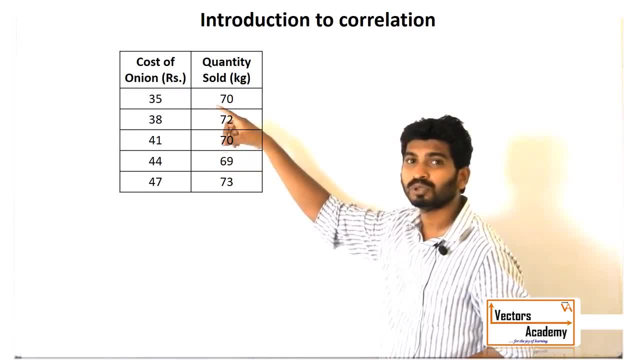 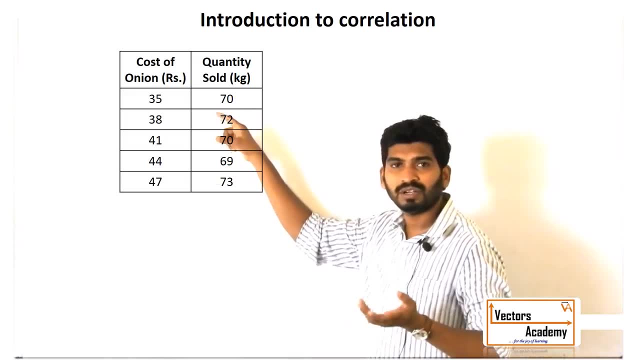 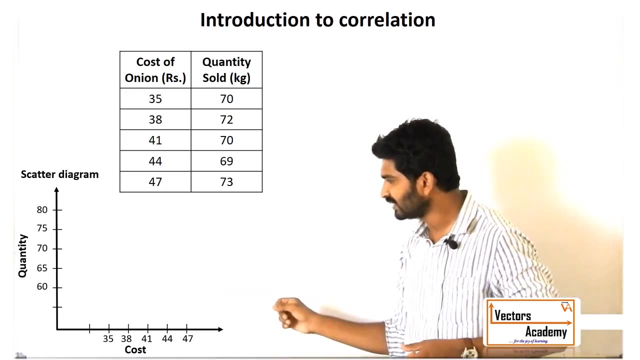 Now, if you see carefully, the prices of onion keeps on varying throughout the year, but the quantity sold does not vary throughout the year. much right. There are few groups whose sale does not depend upon the price. So, again, if I look at the scatter diagram, the x-axis denotes the price. 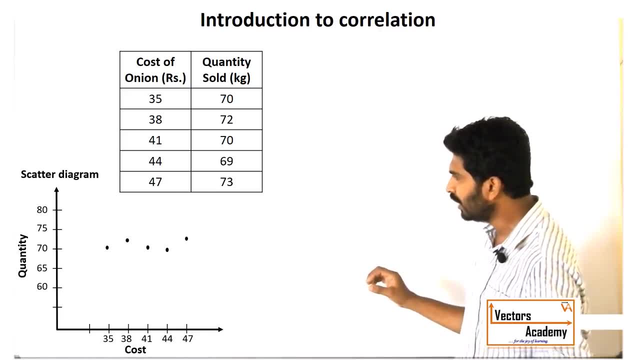 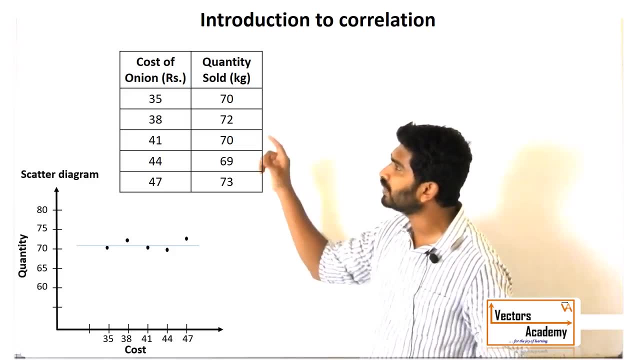 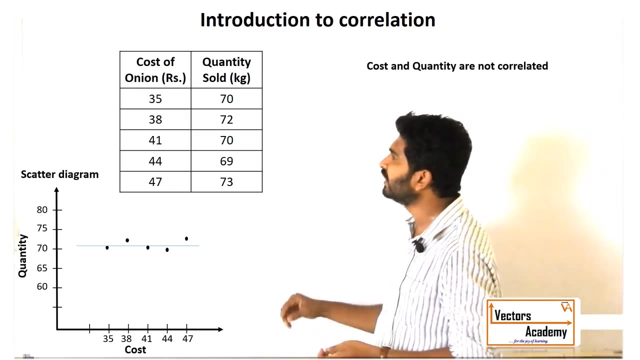 the y-axis denotes the quantity sold. If I look at these points now, you can see that right. So the graph neither increases nor decreases. So I can say there is no correlation between the price and the demand of onions, Got it? So that is exactly what is covariance. There are a few. 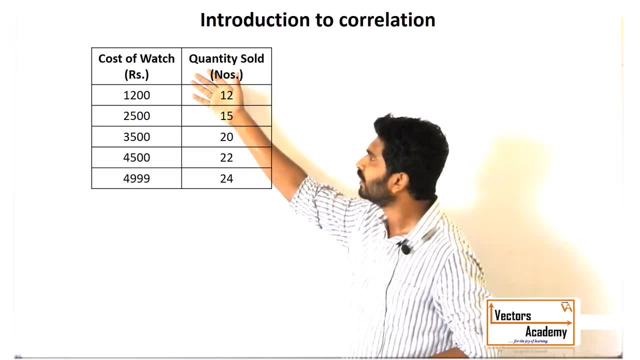 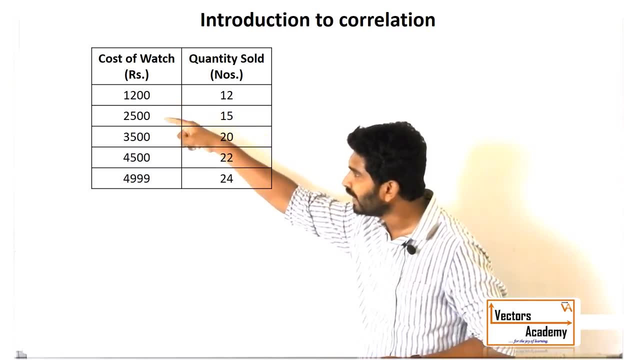 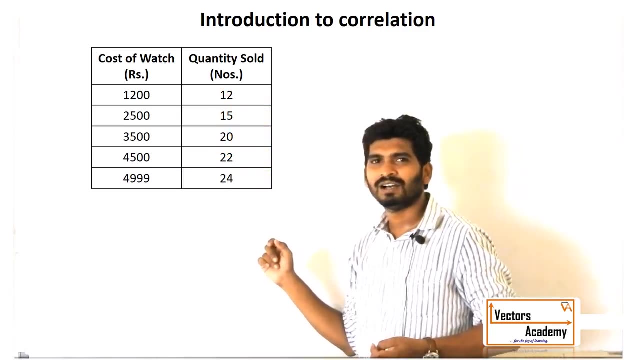 groups such as: okay, these are luxury groups, For the luxury groups. what happens? you can see, the price is increasing, whereas the demand is also slightly increasing. okay, So what happens is, even though the price increases, the customer thinks that the price is increasing, right, So the 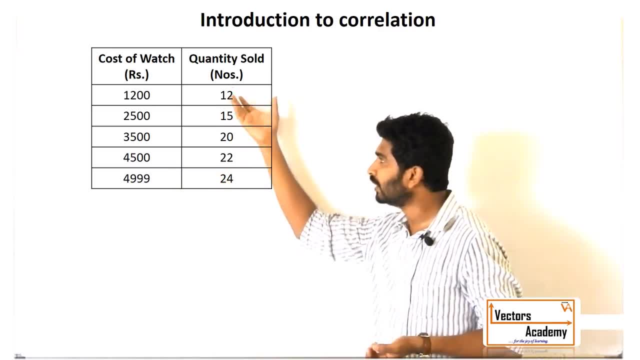 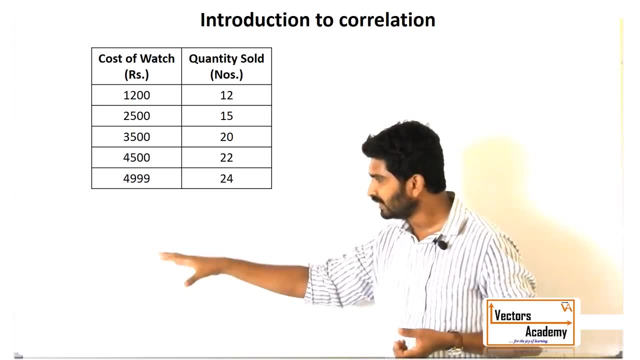 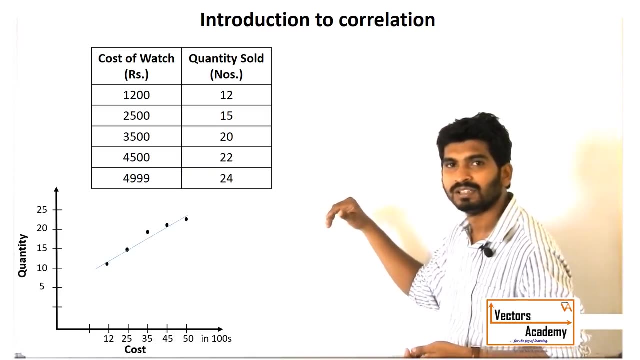 more the price of the product is the luxury product, the higher the quality is And that is the reason why it gets sold more than the other groups. okay, So in this, if you see the scatter diagram, the price and the demand, you can see the graph goes slightly upwards. So I can say: 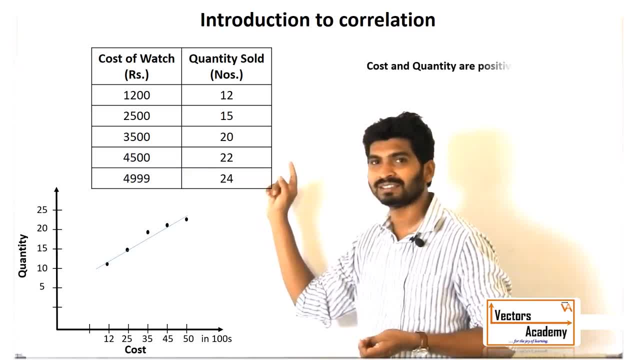 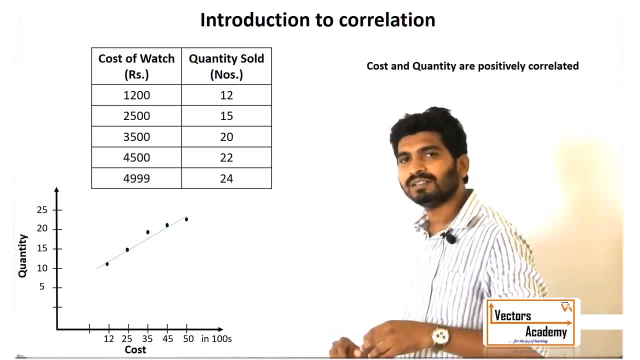 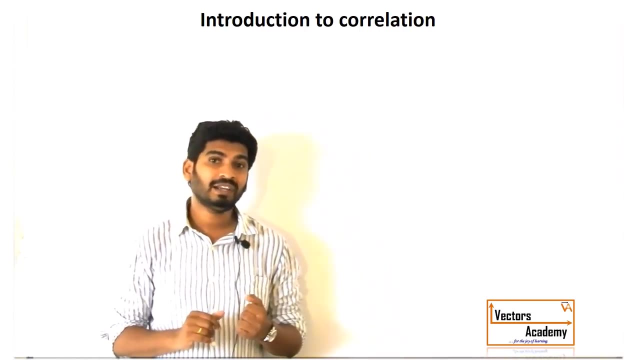 there is a positive correlation between these two variables, the price and the demand. So, once I understood this, now what happened is, earlier the statistician used to use the scatter diagram to explain the correlation between variables, But later on what happened is the statistician had different opinions about the scatter diagram. 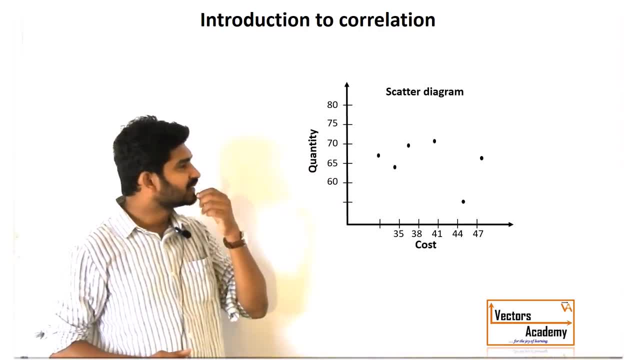 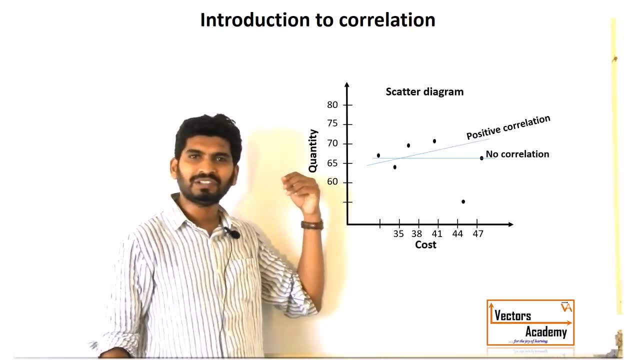 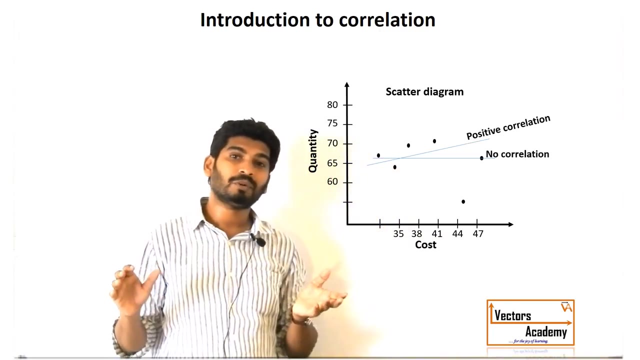 Take a look at the scatter diagram Now. some statistician said the graph is increasing, whereas some said there is no proper correlation between the two variables. Now this problem arises because the scatter diagram does not actually give you a mathematical value to a variable. So what Carl Pearson did, is he? 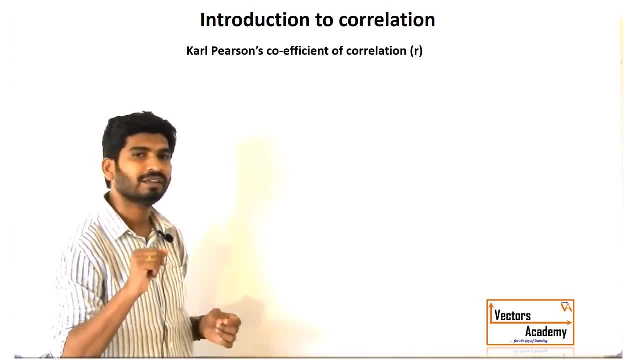 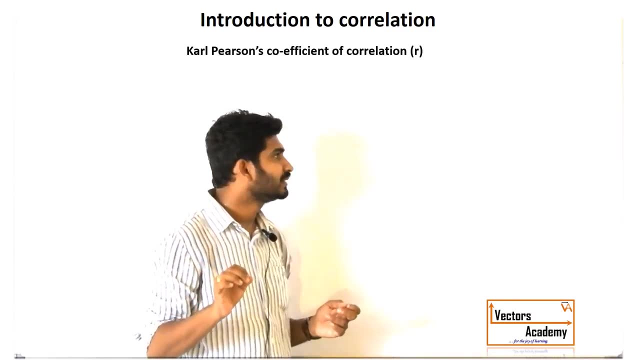 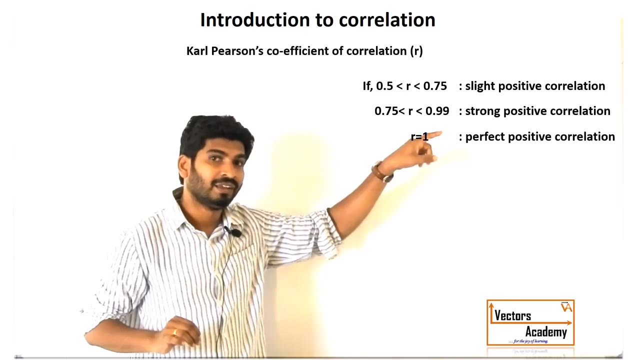 calculated Carl Pearson's coefficient of correlation That actually gave a mathematical value to the correlation. You can see the symbol for this coefficient is r. If the value of r is greater than 0.5, then I can say there is a slight positive correlation. The value of r is greater than.